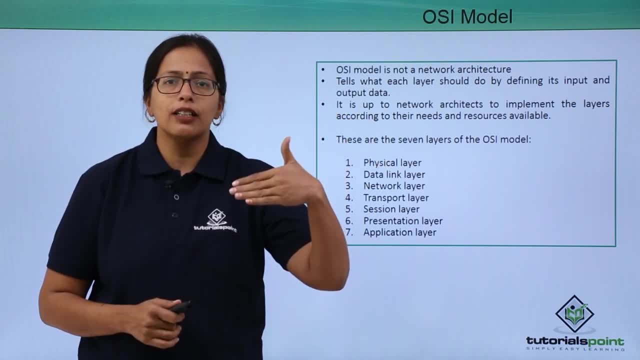 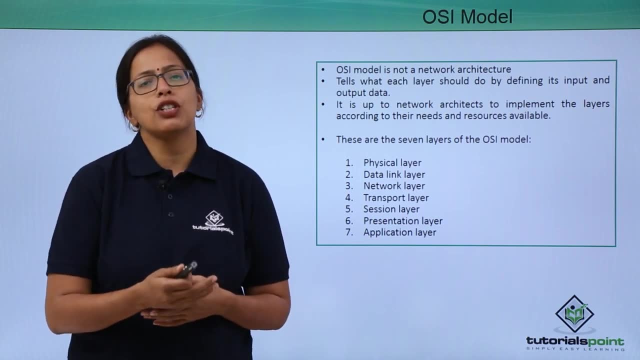 Node 1 is sending a request to node 2.. So node 1 is the client machine and node 2 is the server machine. Now remember that any point of time, node 1 could become the client machine and node 2 could become the server machine. 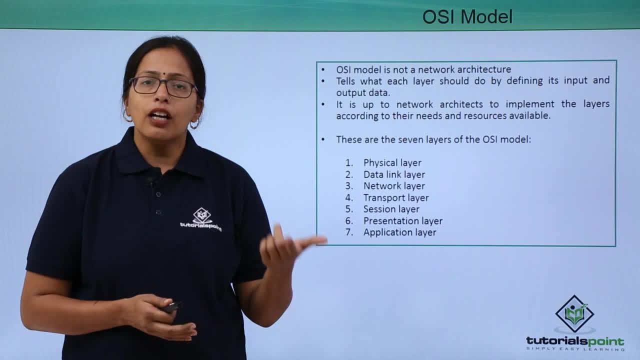 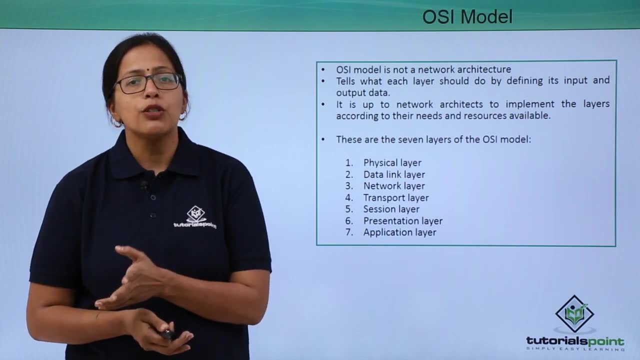 So OSI model is a physical and a logical organization of the network. The network architecture takes care of how it has to be implemented. So let's see what are the different layers of this OSI model. There are 7 layers in the OSI model. 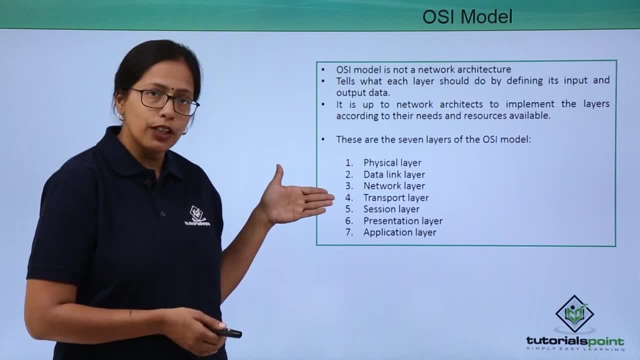 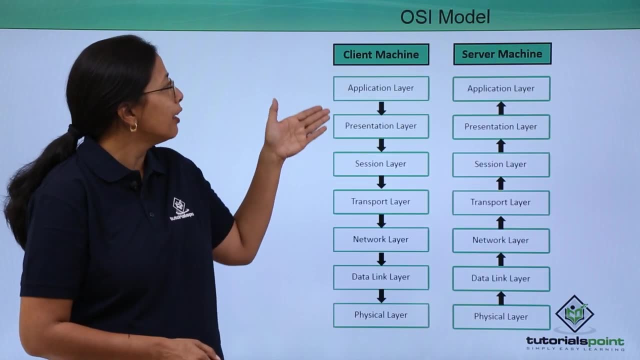 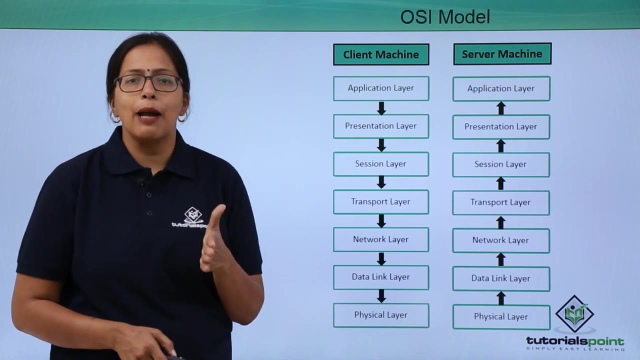 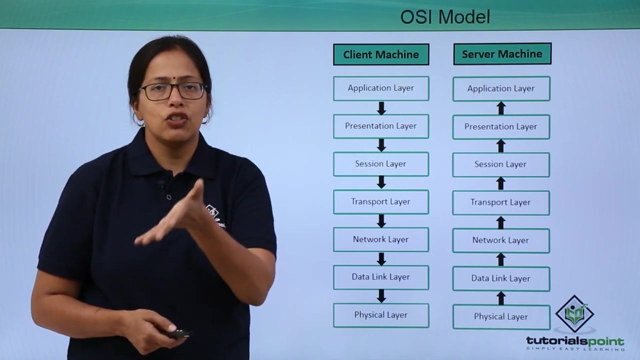 Physical layer, data link, Network layer, transport layer, session layer, presentation layer and the application layer. So let's see how these layers are there at the client end and the server end. First and foremost is the application layer. What happens in the application layer? The client machine is sending a request or it wants to exchange some data, So file chat request or sending or receiving of a video file or a multimedia file. 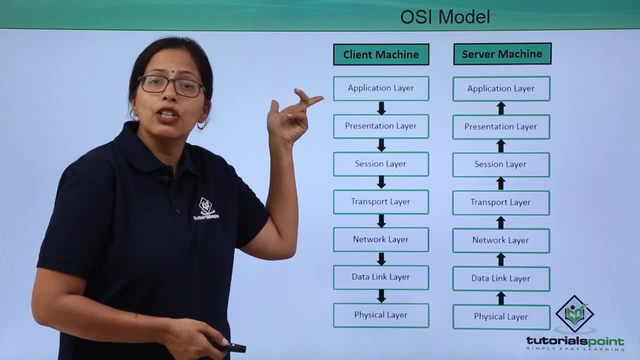 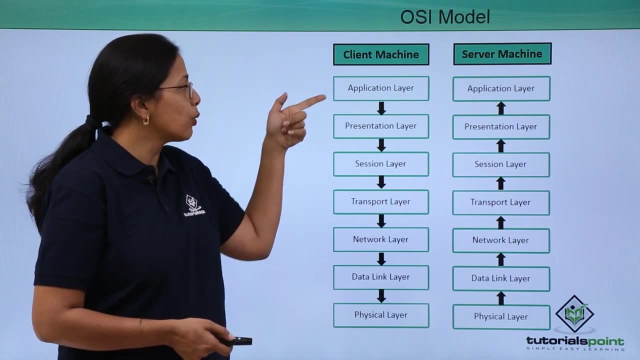 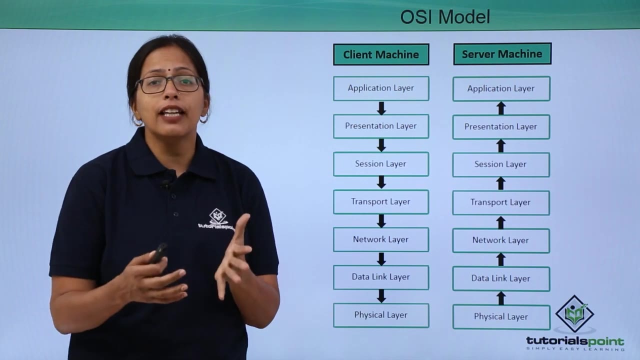 So the file as it is Is there at the application layer. The application layer decides that this can be done or cannot be done and it sends this request or the file itself to the presentation layer. The presentation layer is responsible for presenting that data in a form that is acceptable to the server machine. 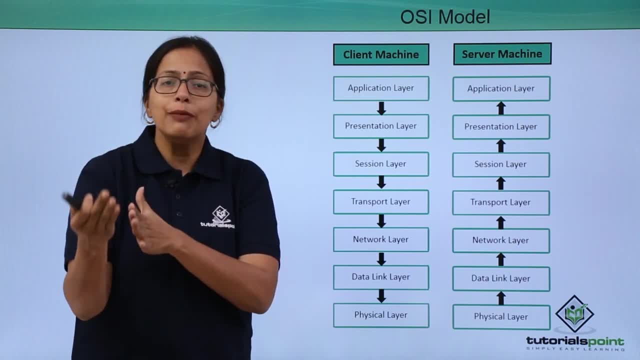 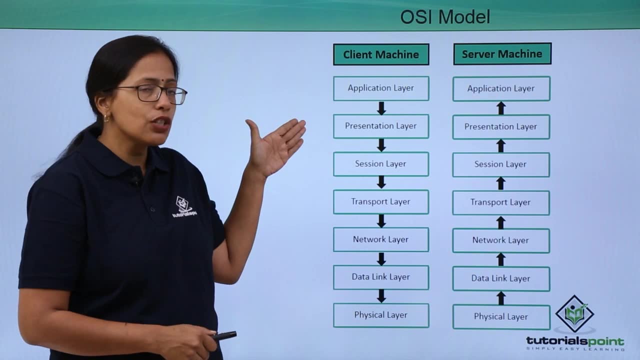 Because server machine has its own configuration, its own limitations of accepting a request, fulfilling a request. So that has to be taken care of by the presentation layer layer. The presentation layer then sends the file or the data to the session layer. What the session? 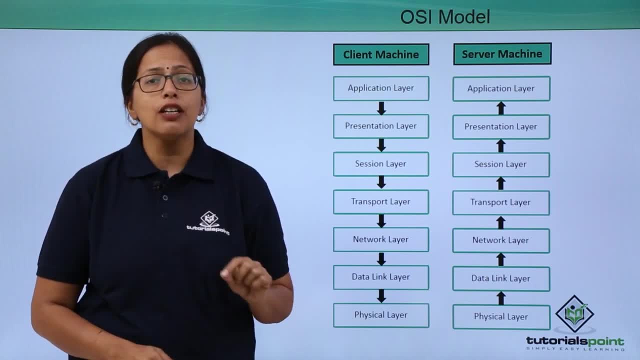 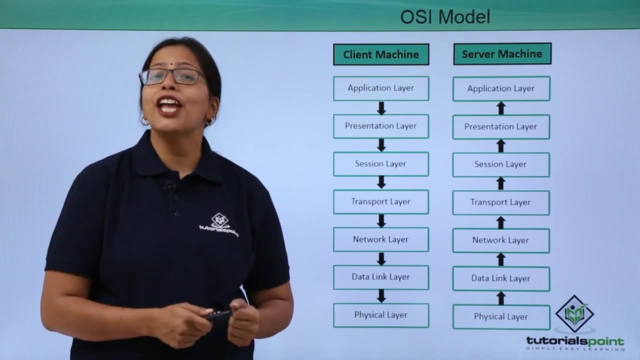 layer does. Session layer is responsible for establishing a session. Say, for example, the server machine is switched off. Can it take that request? No, it cannot take that request. So the session layer will decide whether this request can be fulfilled or not. If it can be fulfilled. 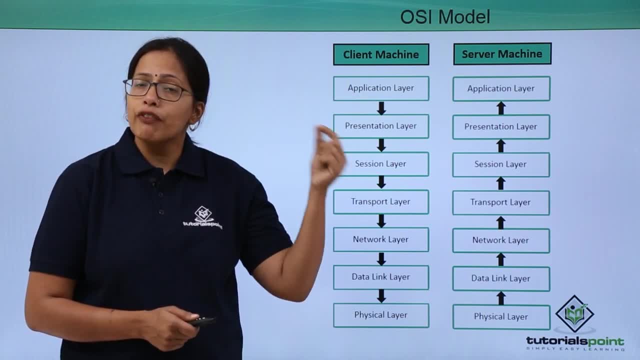 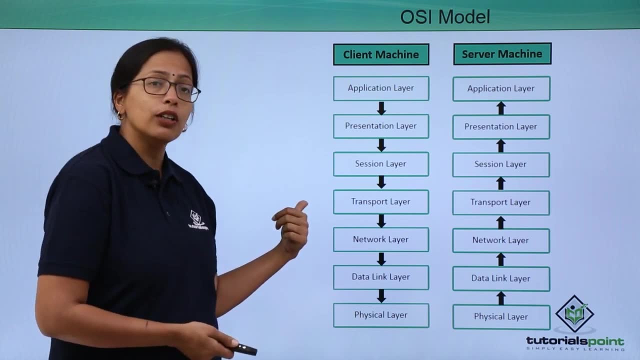 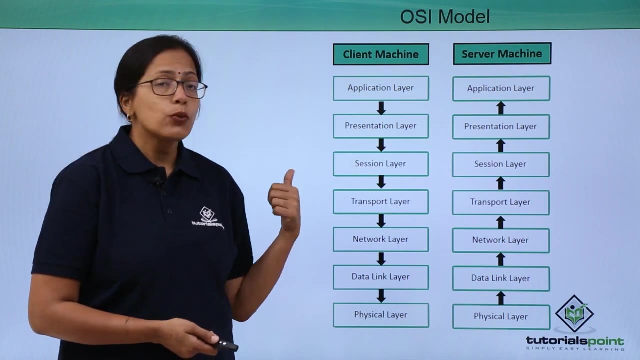 then that session is established. That means the server machine is ready to accept a request from the client machine. The session layer then will send it to the transport layer. Now we have studied in earlier module in earlier videos, that switching technique uses circuit switching or 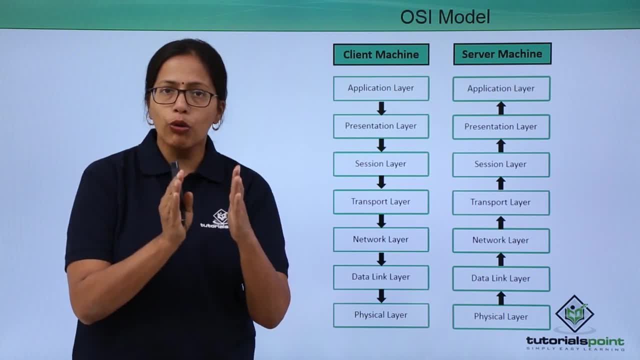 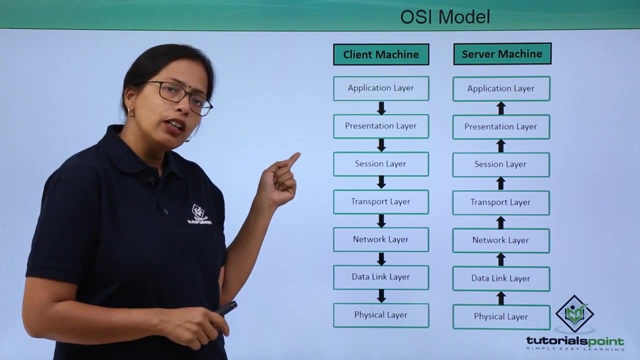 packet switching. In packet switching the data is broken down into different, smaller packets so that they can be sent over the network. Now in the OSI model packet switching is used till the session layer. the file is in its own form In the form. there is a file called packet switching In the session layer. the file is in its own form In the. 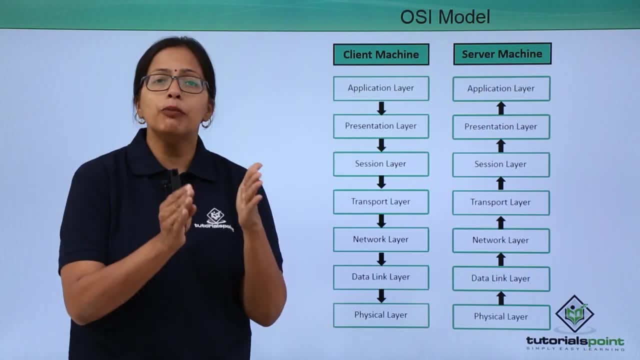 out queroson другой panel citizen file, is entendu, is in its own form now, as in sessa system Case that we want to send at the sessa system case at the transport layout is appropriate. It will be broken down into smaller frames. Trans svib adulti koy test file to be added in corporate. 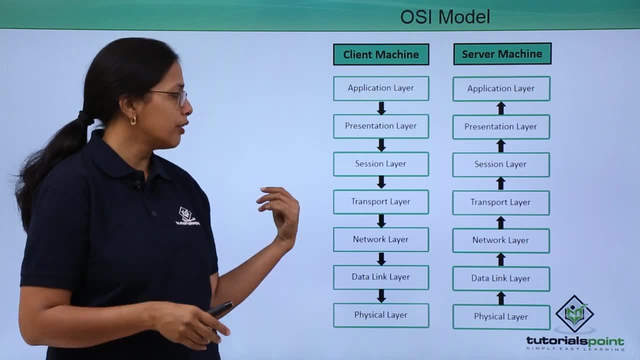 report and shorter time period, Now 6 times higher. alors skill will change the speed. employment per PAREM p shock Partier number to calculate is longize 2 times theAMR of a four time number available data packets. That is what the transport layer will do. What will the network layout do? 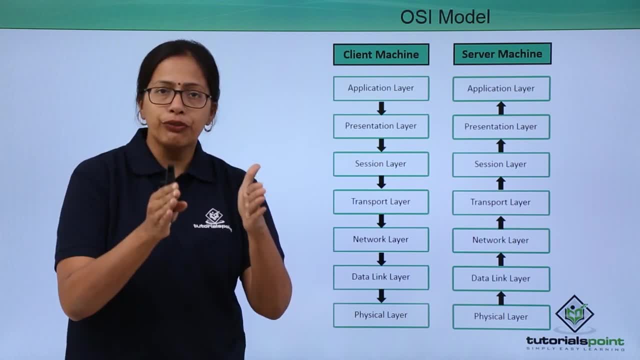 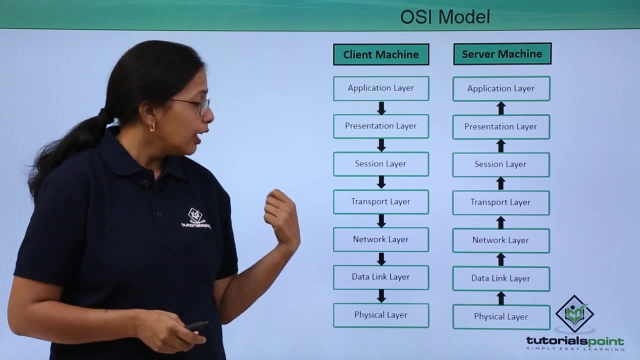 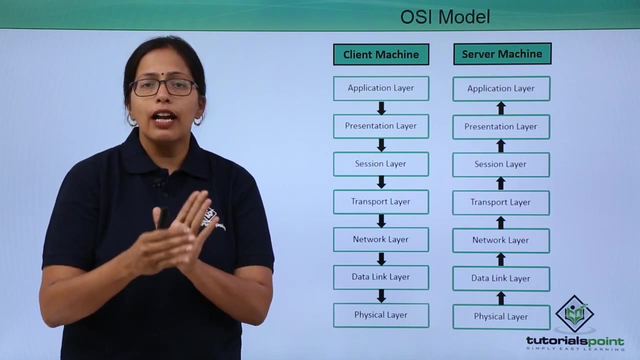 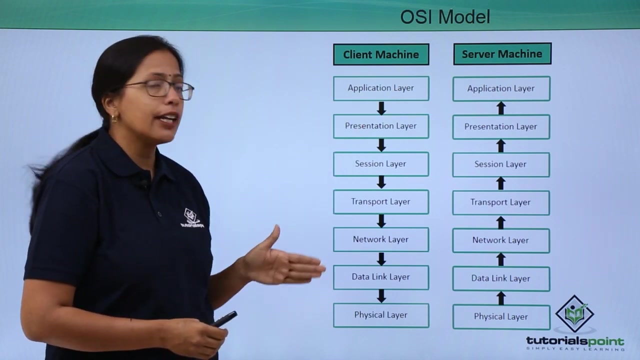 The network layout will break it down into further smaller packets at the source address and the destination address. the network layout are also responsible for attaching a protocol to to it so that it can travel to the next layer or the server machine After the network layer it is. 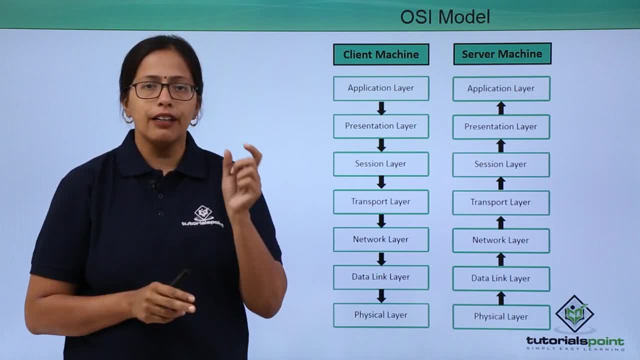 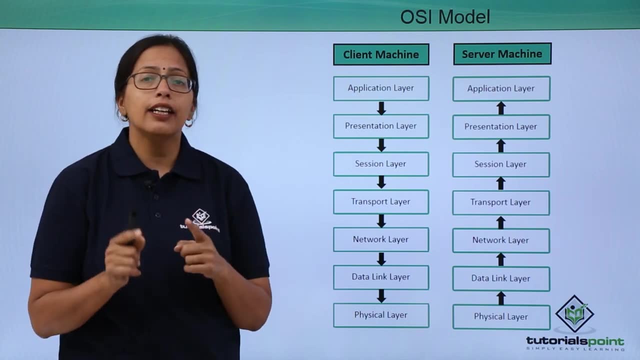 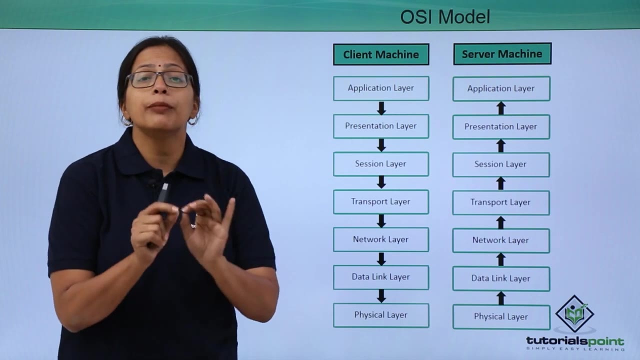 sent to the data link layer. The data link layer has two functions. It will add a start and a stop flag at the end of each datagrams and the data link layer will also check that in the way from application layer, presentation layer through network layer. there has not been any error in. 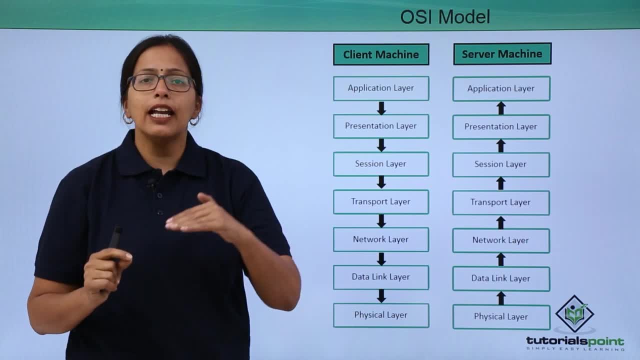 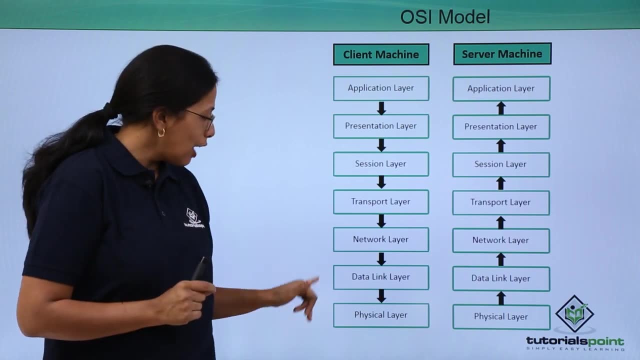 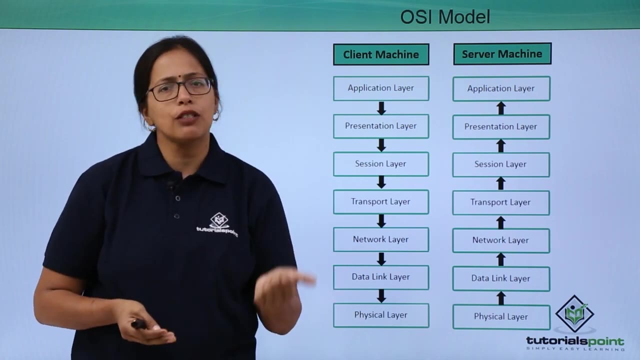 the message. If there has been any message error, then it will ask the upper layers to resend the file so that the correct file can be sent. After the data link layer, it will come to the physical layer. Physical layer is the actual layer where the actual transmission of data takes place through. 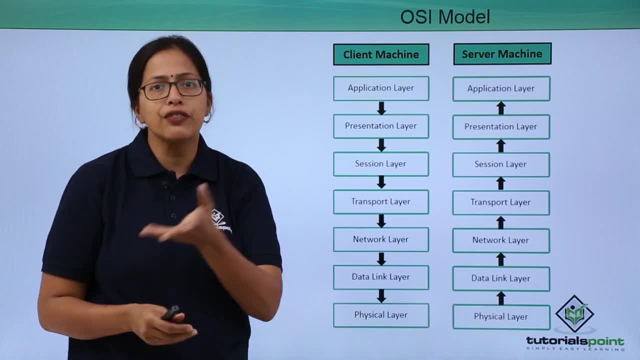 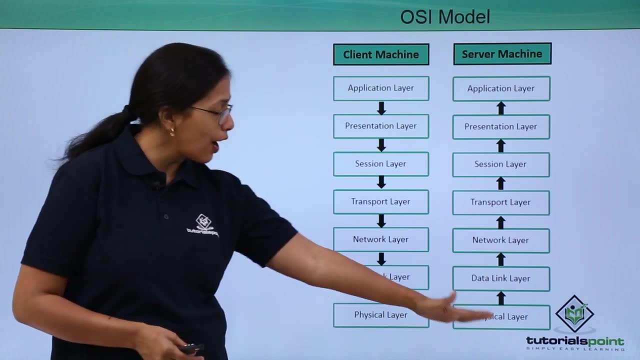 optical fiber cables, coaxial cables, in fact, radio waves, infrared- whatever way has to be there. Now. this is the physical layer of the client machine. Data has started traveling. It will go through the data link layer and it will send the message. If there has been any message error, then 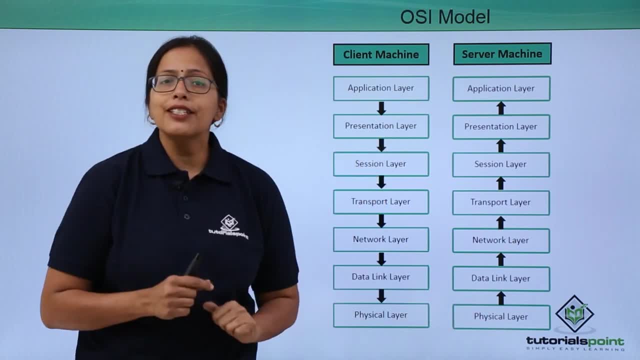 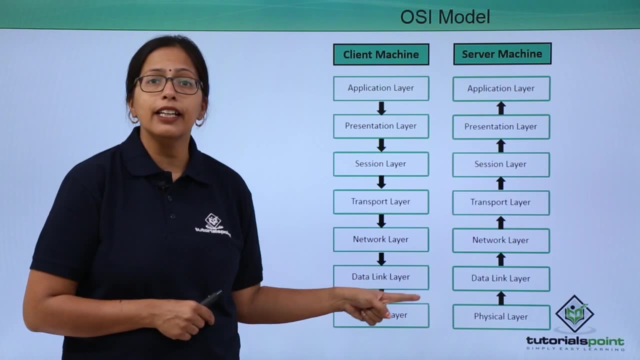 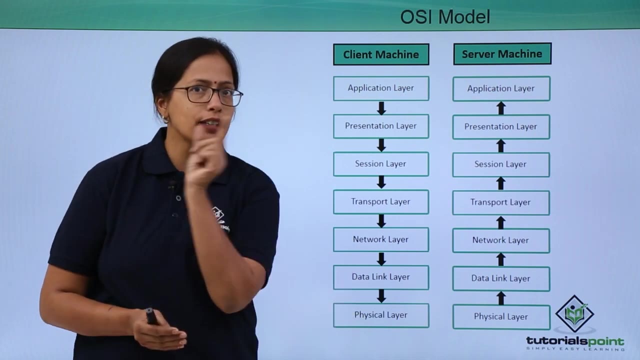 it will go to the physical layer of the server machine At the server end. what happens At the physical layer? the data has reached in the form of bits and bytes At the data link layer. now something opposite will happen At the client level. data link layer was adding a start and a. 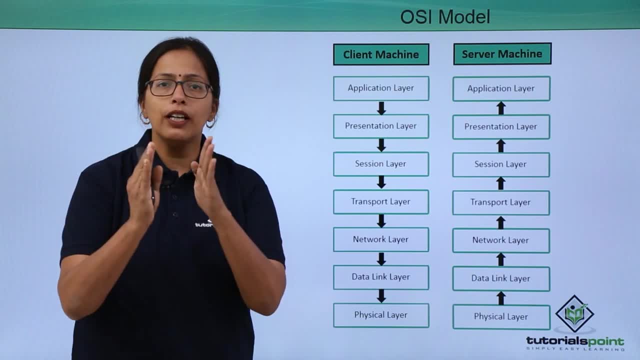 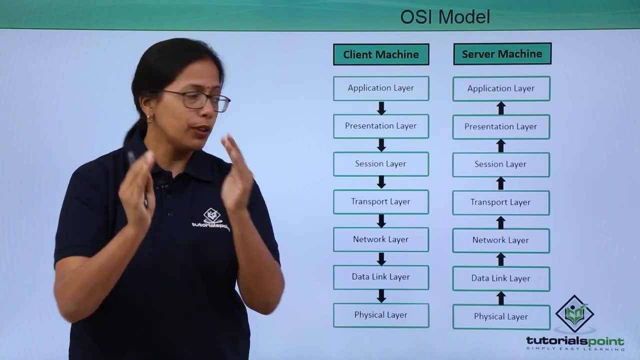 stop flag. Now data link layer of the server machine will take away those At the network layer. what will happen? They will be assembled together because the client machine of the network layer was breaking it down, So opposite to what was being done by the client. 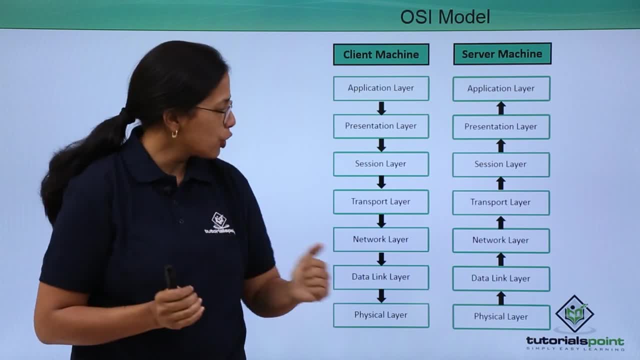 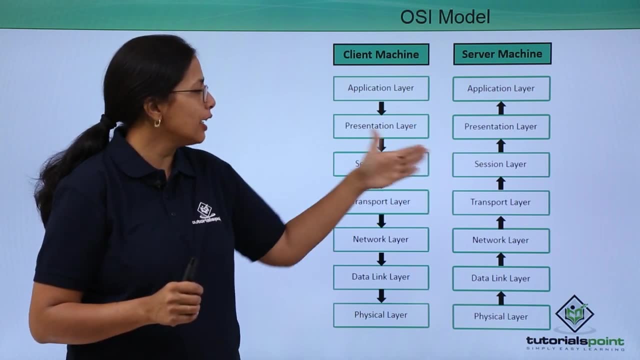 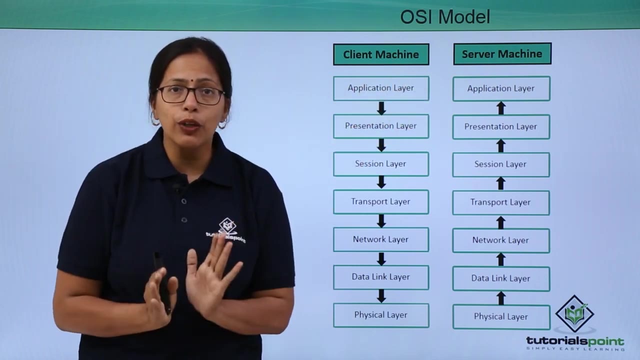 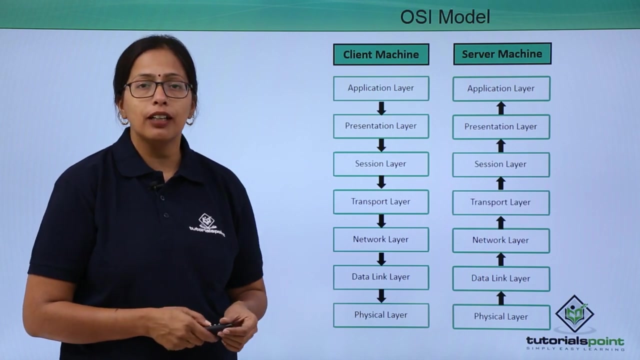 machine levels, the server machine levels, will be functioning Then, at transport layer they will be assembled together- Session layer, presentation layer- exactly opposite to what was being done At the application layer. finally, the whole file will come together in the form that was being sent by the client machine, and that is how the server machine will accept the. 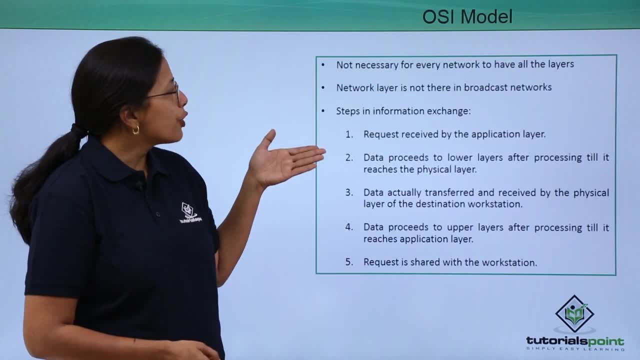 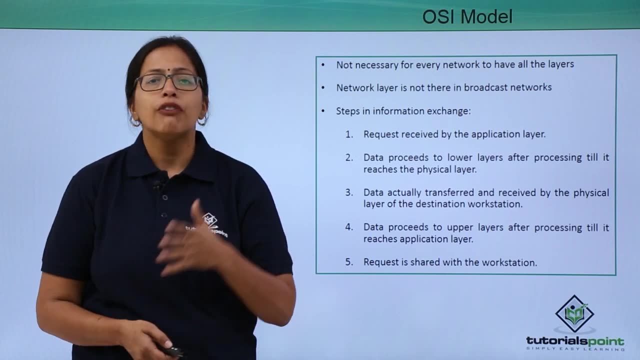 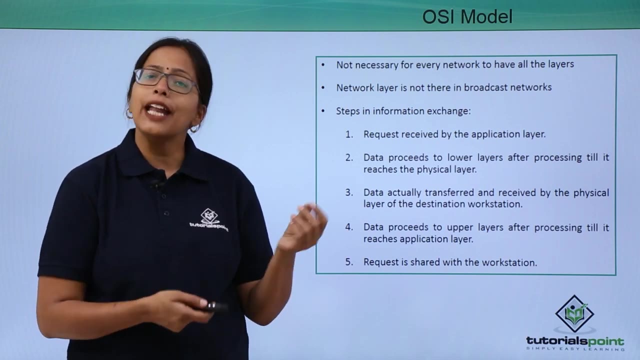 file. Now you should remember that it is not necessary for any network architecture to have all these layers. okay. For example, if there is a wi-fi connection, the wi-fi connection will not need have a network layer. okay, because network layer is concerned about the physical connection, So that 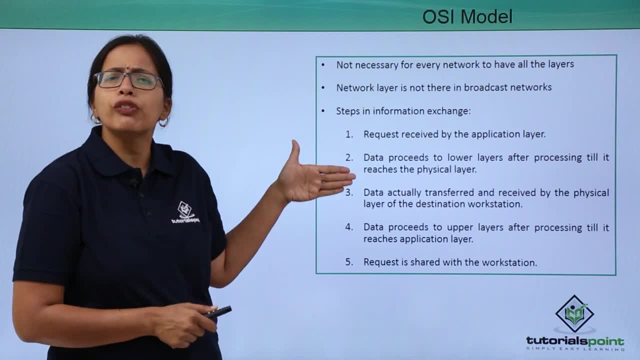 layer will not be required. Now let's just give an overview of what I have told you just now. what are the things that we need to take care of? So let's just give an overview of what I have told you just now. what are the things that we need to take care? 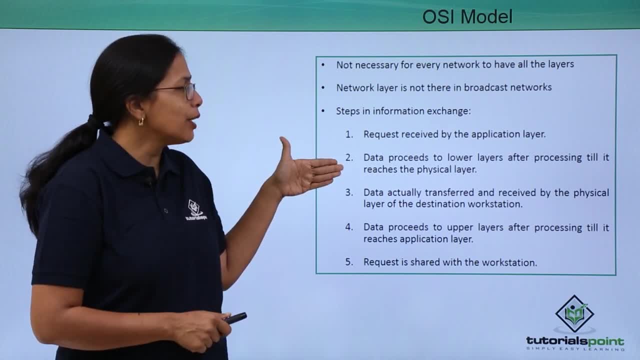 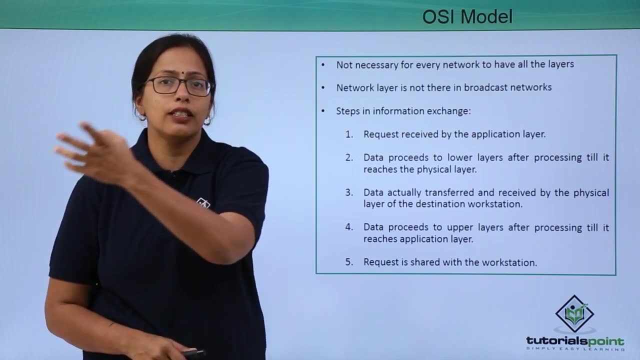 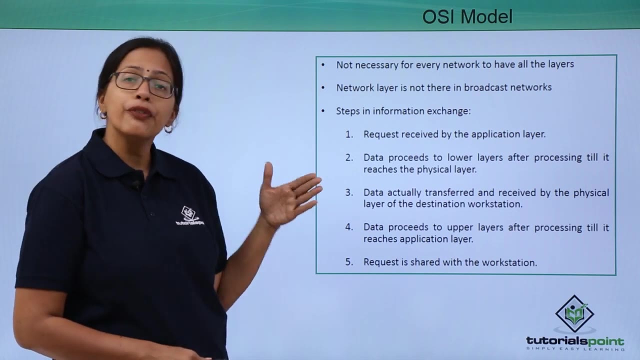 Request is received by the application layer, The data proceeds to the lower layer. after processing, They are breaking it down into datagrams, or they are adding source destination addresses, or they are adding start and stop flags. Data is actually transferred by the physical layer. The physical 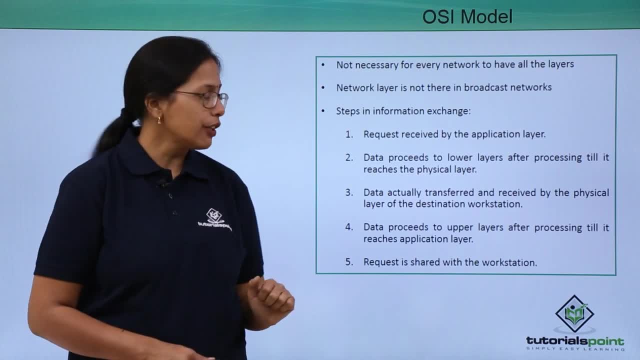 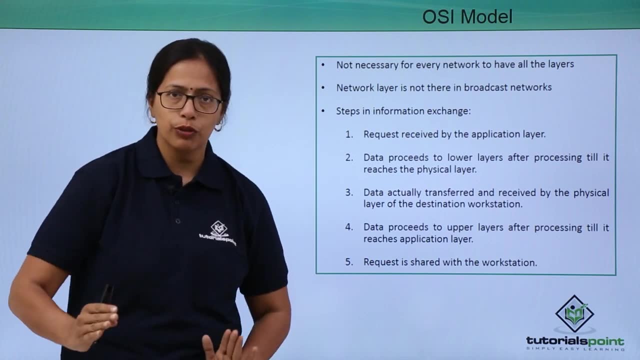 layer of the client machine sends it to the physical layer of the server machine. The data proceeds to the upper layer after processing. So, client machine, it has come down, broken, broken, broken. it will reach the server. it will be joined together, joined together and it will reach the. 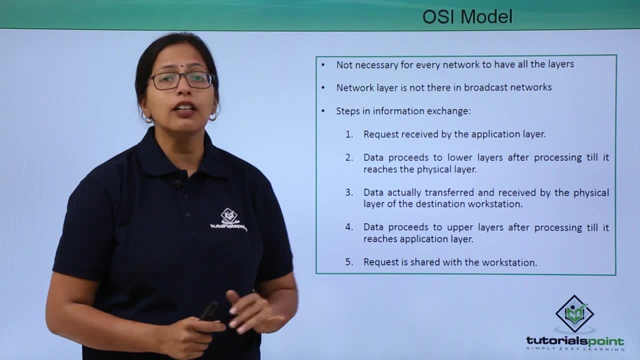 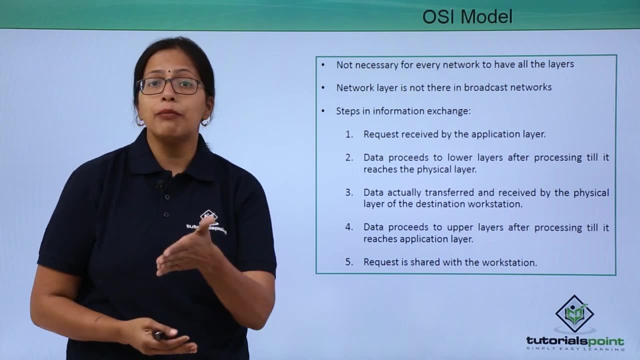 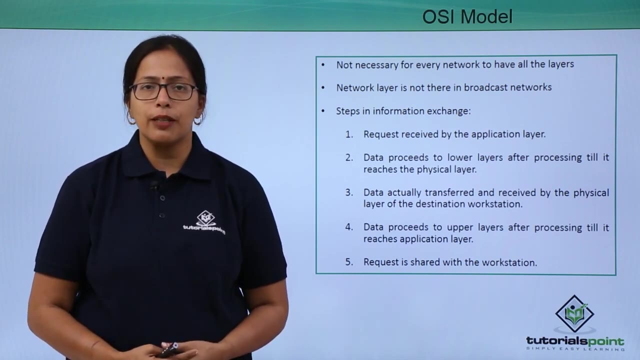 finally, the server machine Request is shared with the workstation. What does this mean? This means that before the actual transmission can take place, the session layer establishes that the server machine is ready to take that request. So in this video we have discussed about the OSI model. 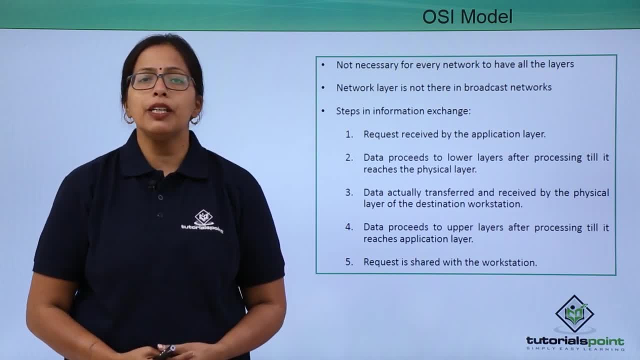 In our next video, we are going to discuss about the TCP IP model.